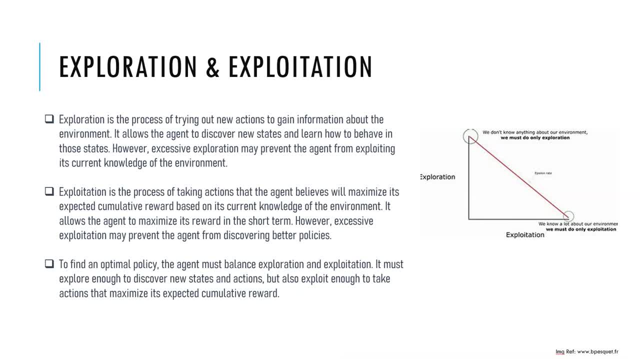 may explore different moves to learn you know about the board position and their consequences. However, as the agent learn more about the game, it may start to exploit it knowledge by choosing the move that it believe has the highest probability of leading it to win. If the agent only exploit, obviously it may get you know stuck in suboptimal policy If it never tries out new action that could lead to you know better. 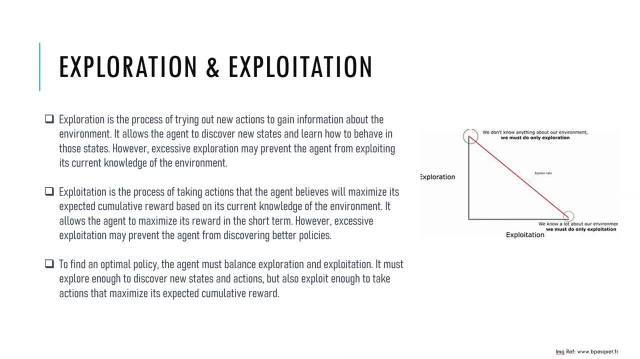 policy? obviously it will, you know, get stuck in the suboptimal policy. So, on the other hand, if the agent only explore, it may not be, you know, able to make progress toward finding the optimal policy. Why? Because because you know, if it just exploring, I mean, it doesn't you know understanding which one is optimal policy. obviously it will, you know it is a never ending process, right, I mean exploring. 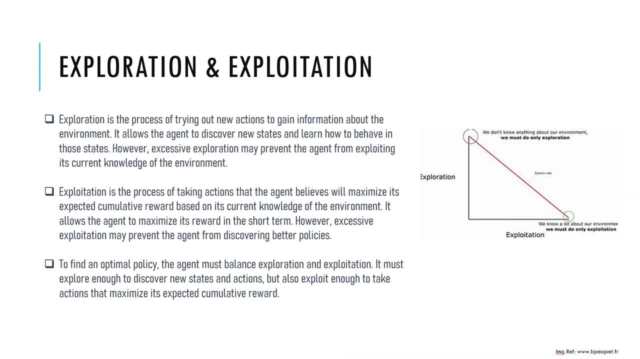 exploring, doing nothing, So so, so therefore, it is important for the agent to you know, balance exploration and exploitation to maximum its cumulative reward over time. Now let's understand trade off between them- how to basically understand the trade off, and I mean how to make them better, Okay, so before that, let's let me give you a real life example. So suppose you, you are at home and you want to go to school, okay, And 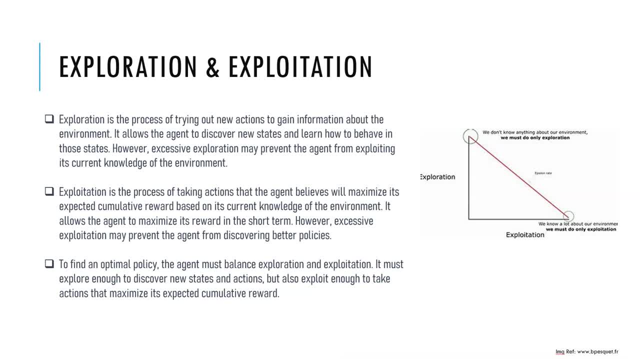 obviously there can be many. you know different path to basically reach your school, right. So let's say you never explored your area, right? So so will you get to know what is a shortcut or, in this term, in the reinforcement term, the optimal policy to reach, you know, a school or home, No right? Obviously you have to explore your area. then only you will get to know. 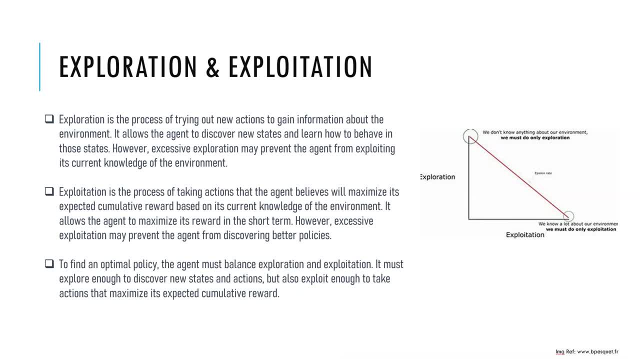 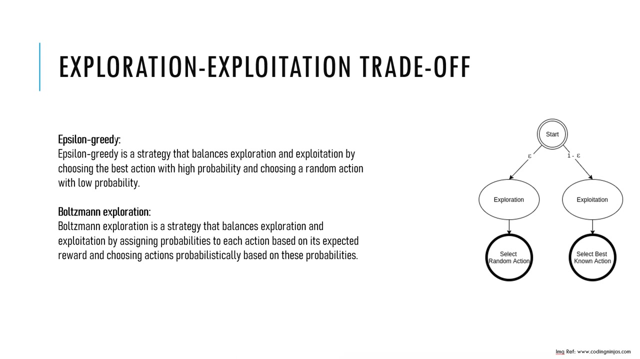 what is the optimal policy? I can have right. Or you can say shortcut: I can get to home, either school or home, right. So this way, the exploration and exploitation. it is necessary to have a balance in between them. Now let's understand what is the trade off between them. Okay, So exploration and exploit, exploitation trade off in in reinforcement learning- this referred to. 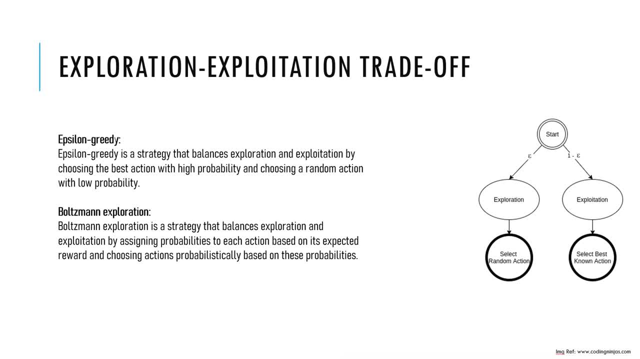 the balance between trying out new action- that is, exploration, or to learn more about the environment, and taking action that agent believes will maximize its expected cumulative reward, that is, you know, exploitation. So as in so the agent must find a, you know, balance between these two term to maximize it cumulative reward over time. So there is two way to do it. One is epsilon, greedy, Another one is bold, when exploration okay. 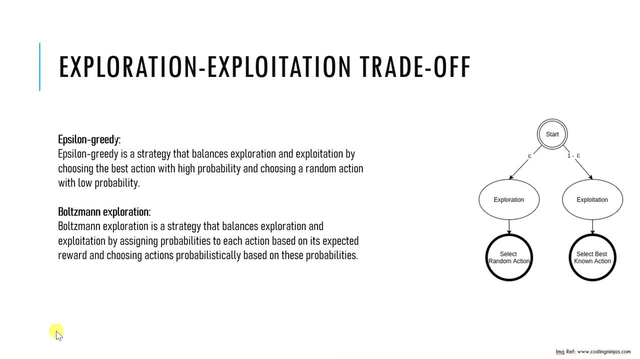 Okay, So in bold, when exploration what happens is, it is a, you know, strategy for balancing exploration and exploitation in reinforcement learning. So it worked by assigning a probability to each action based on the expected award and the you know, choosing action, you know, probabilistically based on these probabilities. So the temperature parameter control the degree of exploration versus exploitation. 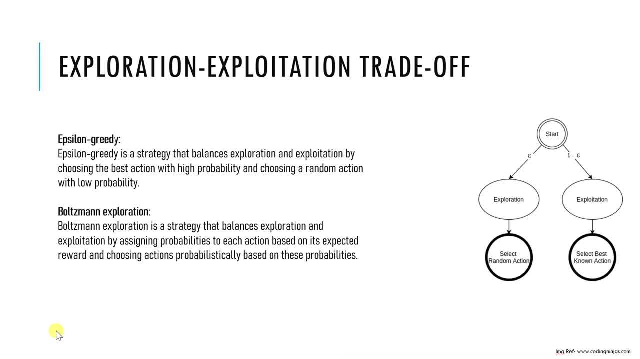 With temperature, with higher temperature leading to more exploration. And this way I mean you can, you know, understand the bold when exploration. Now, other one is epsilon greedy. So epsilon greedy is a simple strategy for balancing, you know, exploration and exploitation in reinforcement learning. So it worked by taking the action that has maximum, or you can say highest expected award, with the probability one minus epsilon. 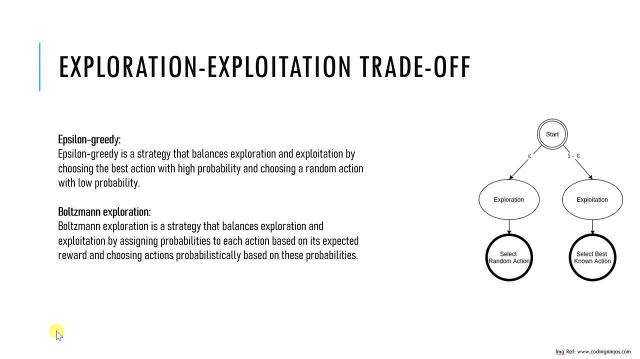 And you know, taking the random action, with probability, epsilon, the parameter of epsilon, will control the, you know, degree of exploration and exploitation. We'll see in example these all term also, And obviously the higher value of epsilon leading to more exploration. So obviously, most of the time you will see that we set our epsilon value to either 0.7 or 0.8, so that it you know, so that we should be able to control the degree of exploration and exploitation. 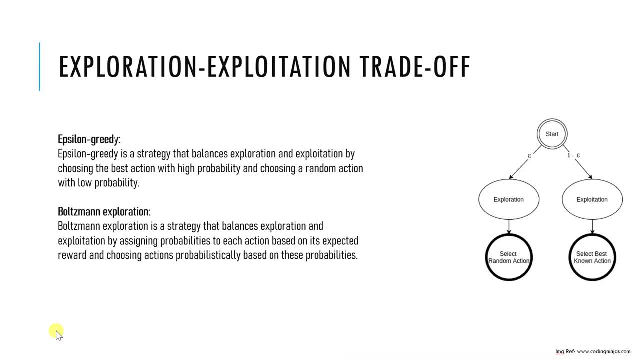 should make a balance in between them. okay, so now what is the difference between these two epsilon, greedy and Boltzmann exploration? so in both of them, the agent balances exploration and exploitation by taking action that have highest expected reward right and occasionally taking random actions, actions or like- or you can say- less likely actions to gain more information. 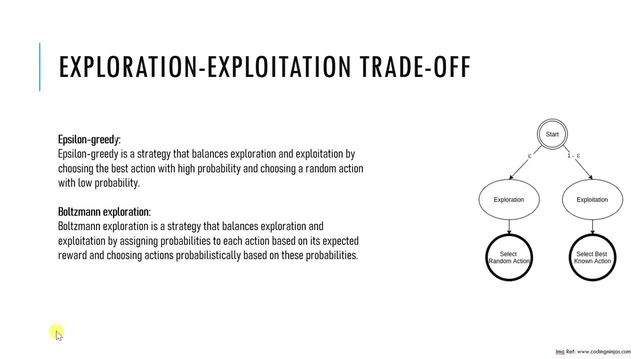 about the environment, but in general, this is not in in the case of a real life situation. right, in most scenarios, you would be, you would, you know, explore only a small fraction of all the possible action, because you don't know all the actions right. so so you have a. you know, in your area there can be you. 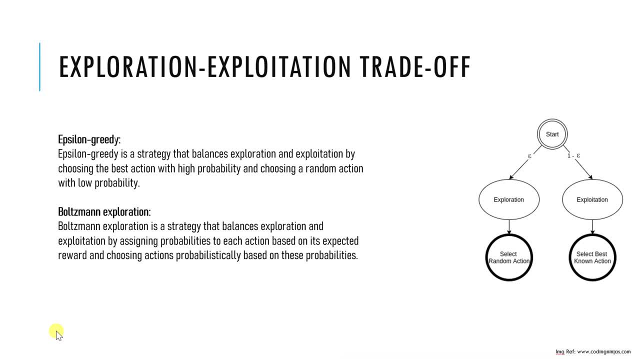 know multiple, you know n number of schools, right. so after reaching one school, obviously you will not going to explore the environment, but in general, this is not in the case of real life situation, right? in most scenarios you would be, you know, explore only a small: the second third, one, right? or you will explore the second third, but you will. 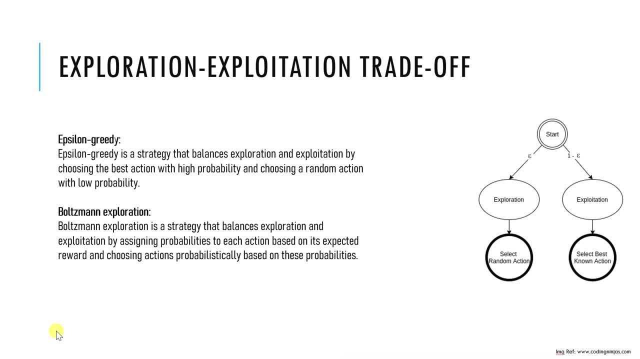 not explore the fifth, sixth, one, right, and that is what basically I am telling. so in real life situation, you will not going to know how many you know possible actions you have. you will only get to know about small fraction. okay, so let's say what, if they there exist, an action there can get, that can get you a lottery. 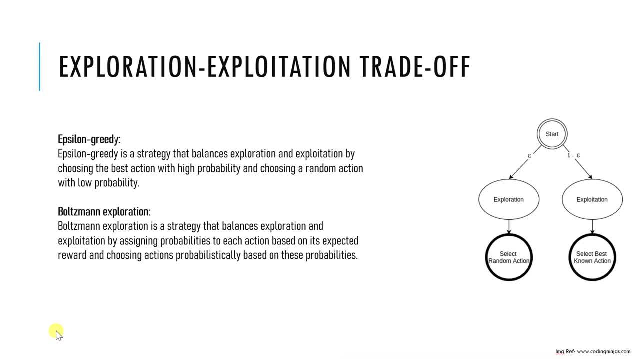 so wouldn't you go exploring more? but obviously at this time you also don't know. I mean, don't want to lose out the benefit of current action right in in case you don't find good option while exploring. obviously, and this is all our real life situation, because in real life situation you only know few schools. but 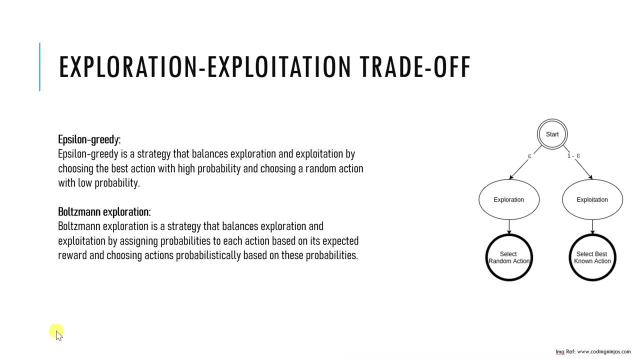 but obviously in, in, in any in your area there can be you know n number of school, but obviously in in any in your area there can be you know n number of school, but obviously after you know finding the best one, let's say the second or third. 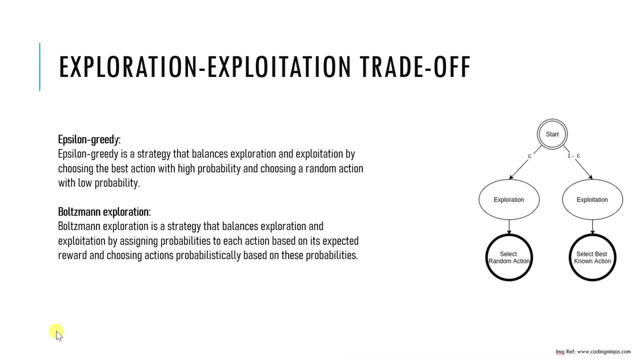 one, you will not going to explore the fifth or sixth one, and that is what exploration and exploitation tells us about. so once we have, you know, accumulated, the best reward will get to take that action, and this is what this exploration and exploitation tells us. okay, hope you understand, understood the terminologies and went to use. 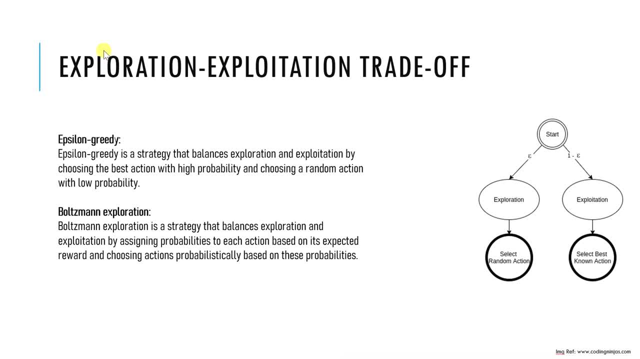 what and what percentage of you know epsilon you will be choosing. okay, so little. so in the next tutorial we will be learning about Markov state. okay,